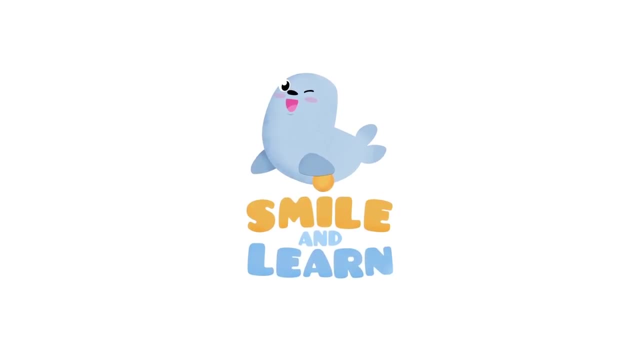 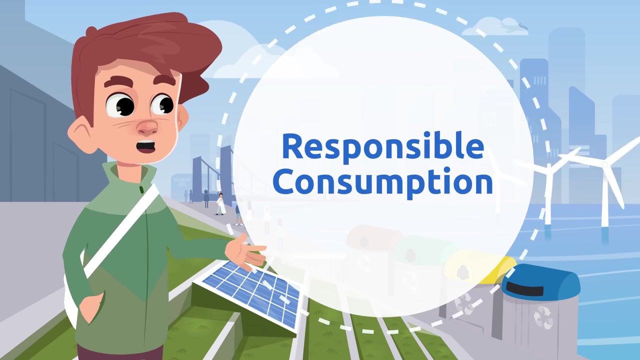 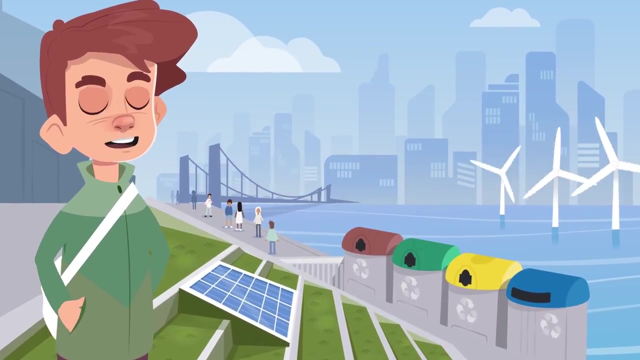 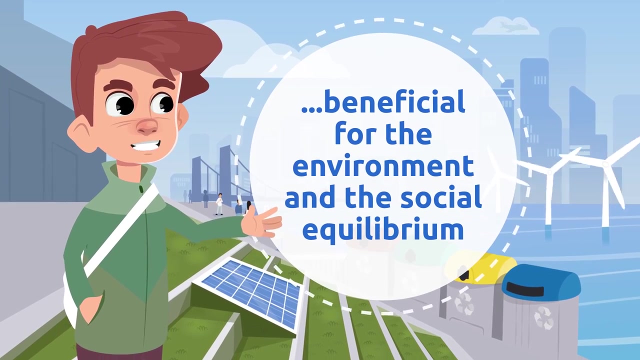 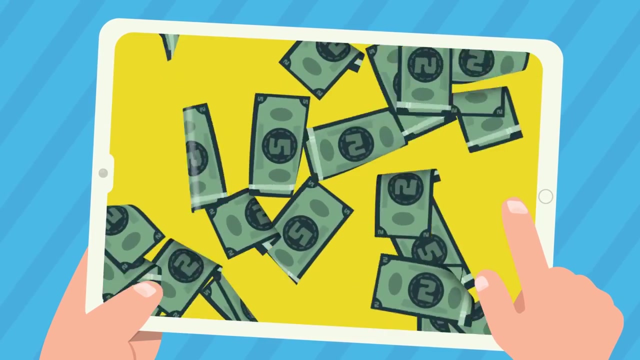 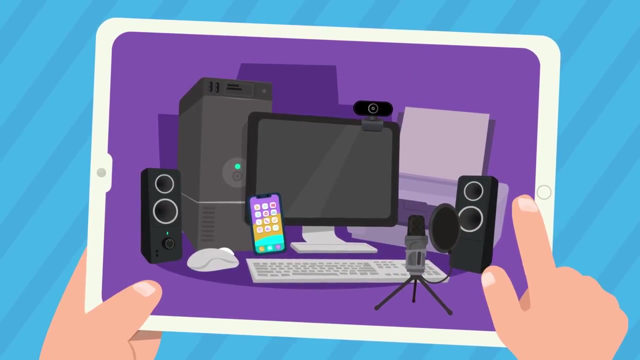 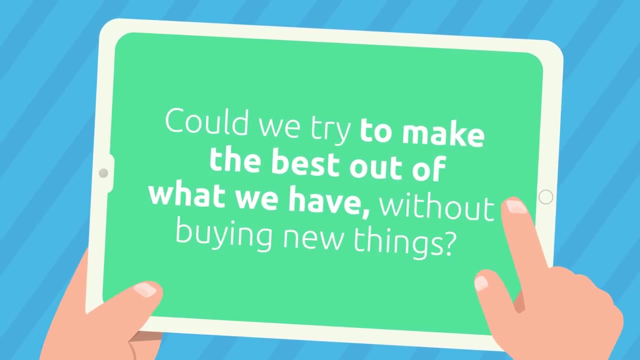 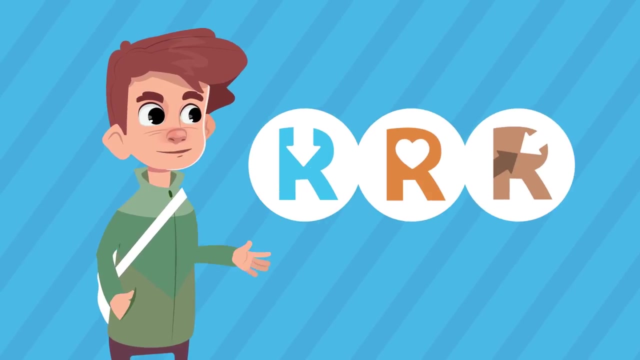 Smile and Learn. Do you think we really need all these? Could we try to make the best out of what we have without buying new things? Responsible consumption is based on the 3R principle: Reduce, reuse and recycle. Look at this shopping basket. 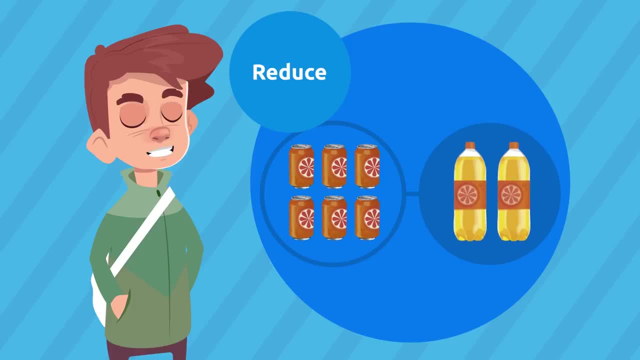 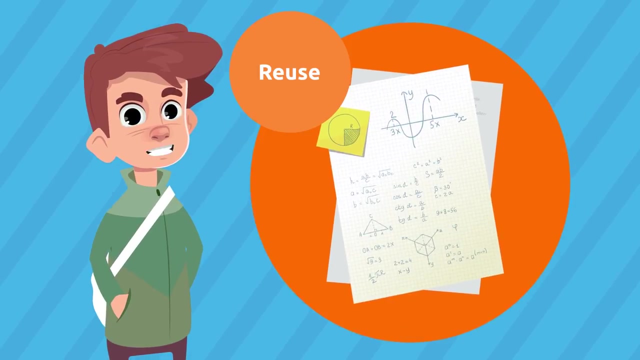 We could reduce waste buying two big bottles of this drink instead of six small cans. We'd be buying the same product, generating less waste. We can reuse this glass jar to store some other foods. We could also reuse these sheets of paper for note-taking by writing on the blank side. 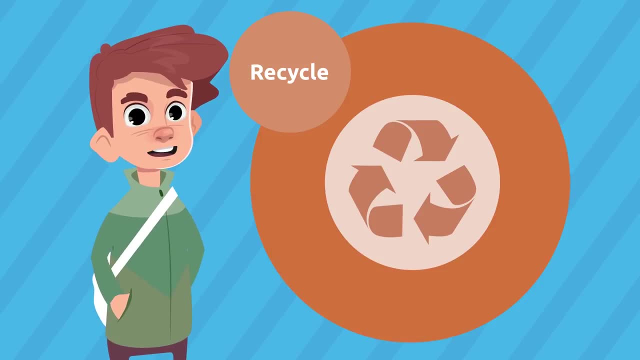 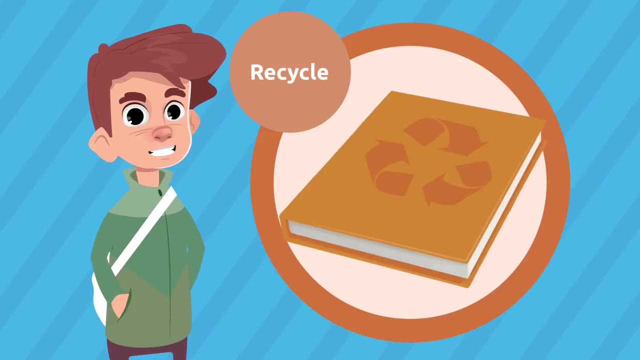 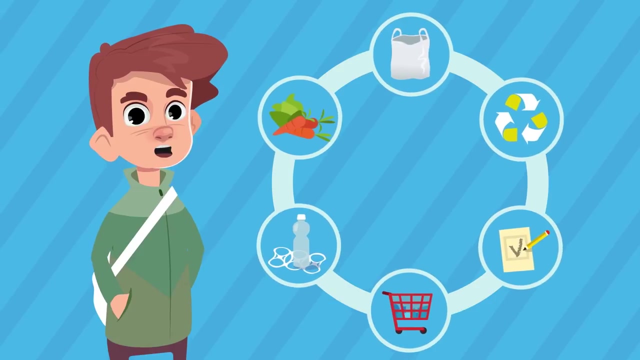 The last step is to recycle. We can recycle material like plastic, glass or cardboard. Did you know? we can make a book by recycling eight cereal boxes? Consuming products we don't need can be very harmful for our planet. That's why we should change some of our habits. 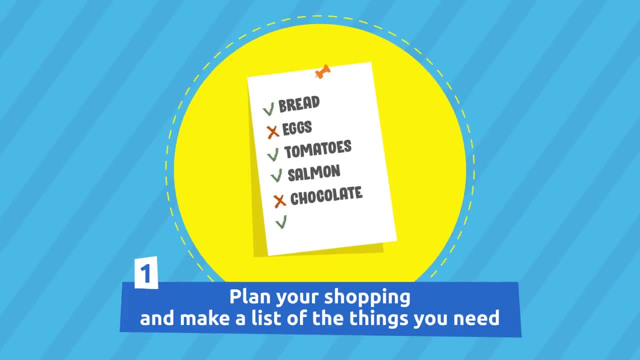 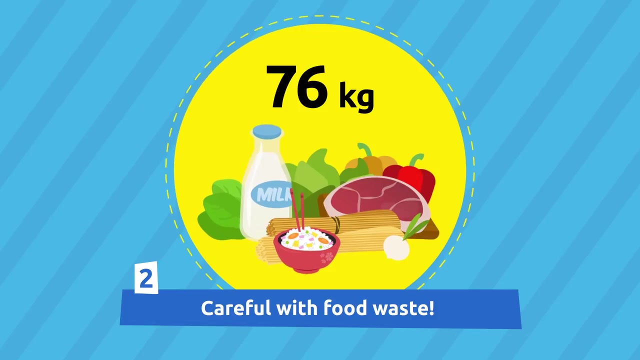 These are some ideas. Plan your shopping and make a list of the things you need. This will help you to save money and keep you from buying products you don't need. Careful with food waste. Did you know that each household weighs .76 kilograms? 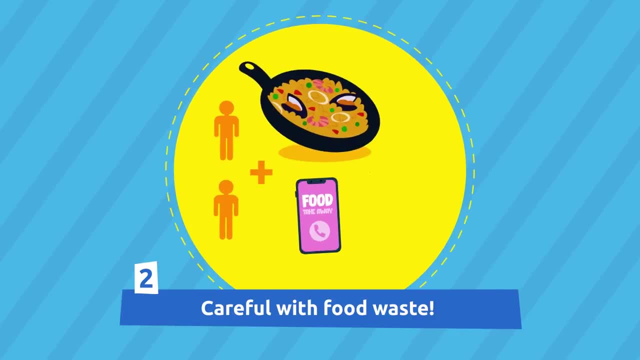 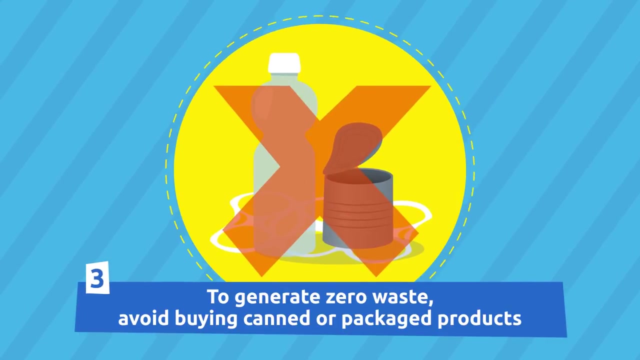 To stop this, it is necessary to prepare or order only the food you'll actually eat. Like we said before, planning your grocery shopping is key to stop buying more than you need To generate zero waste. avoid buying canned or packaged products. If that's not possible, try to buy products packaged in containers that you can reuse and recycle. 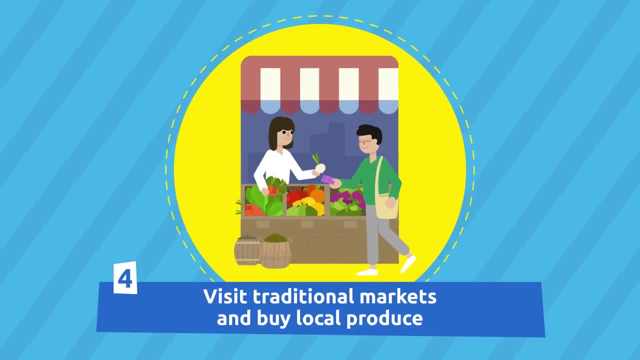 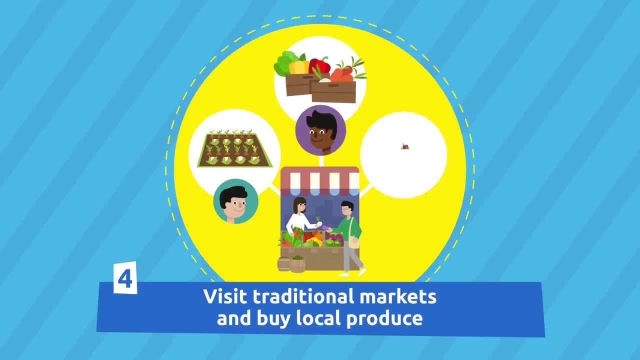 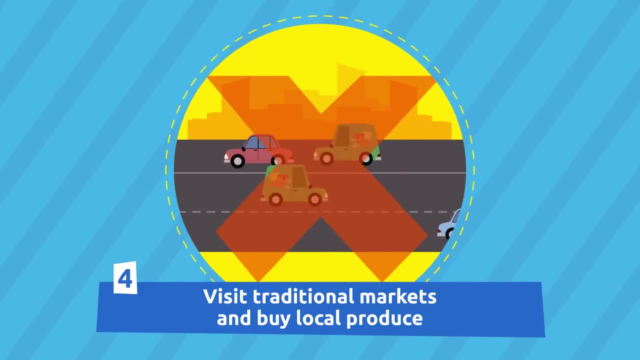 The people who sell at these markets buy products locally. That's why they are more fresh and sustainable. Besides, there's no need to drive to your local market. Besides, there's no need to drive to your local market. You could walk there.